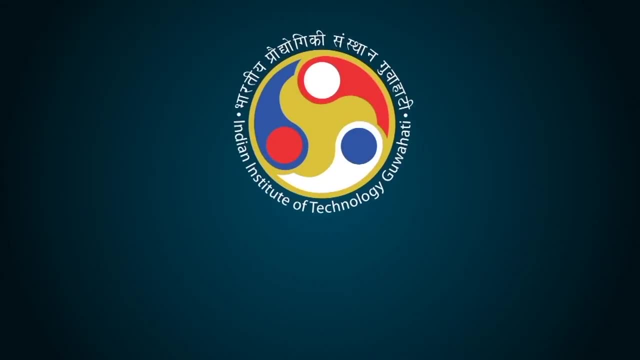 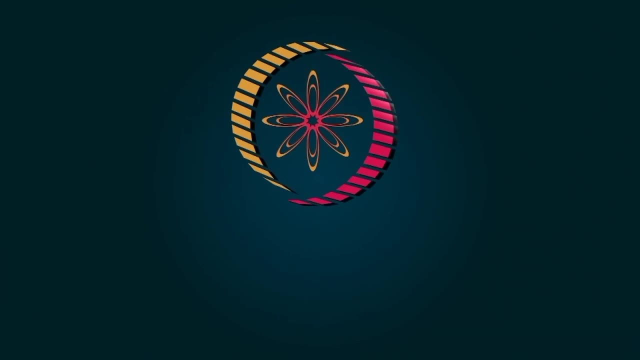 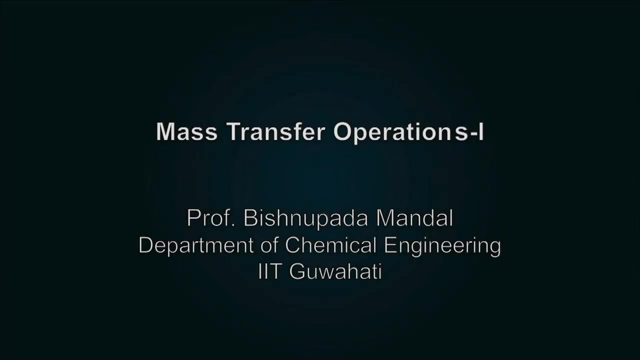 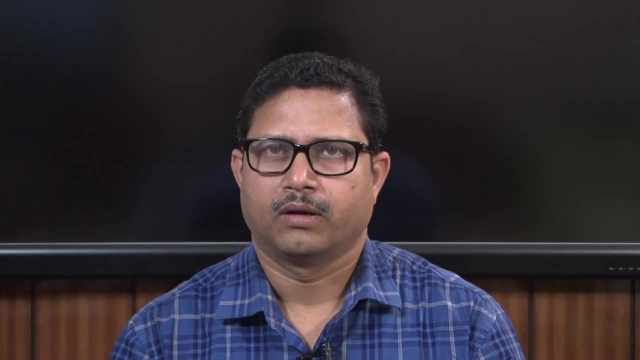 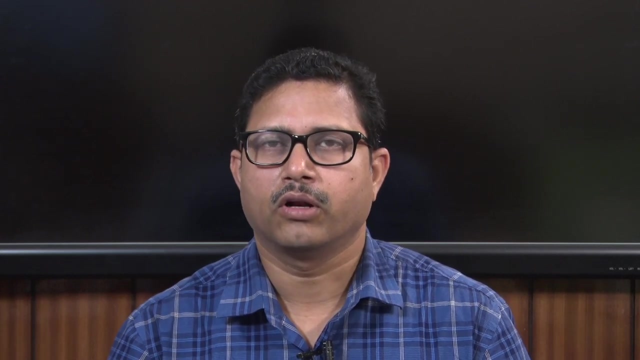 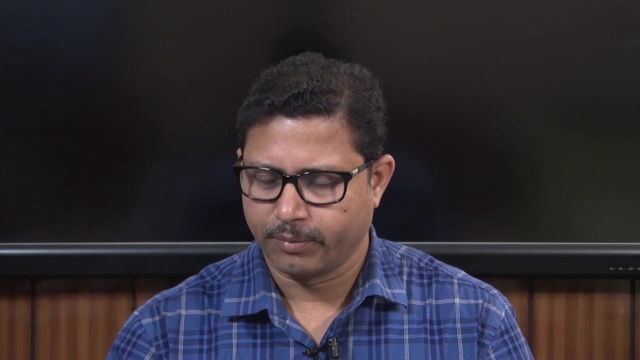 Please subscribe to the channel and press the bell icon to receive notifications when new videos are uploaded. Welcome to the fourteenth lecture of module five of mass transfer operation. In this module, we are discussing distillation operation. Before going to this lecture, let us have 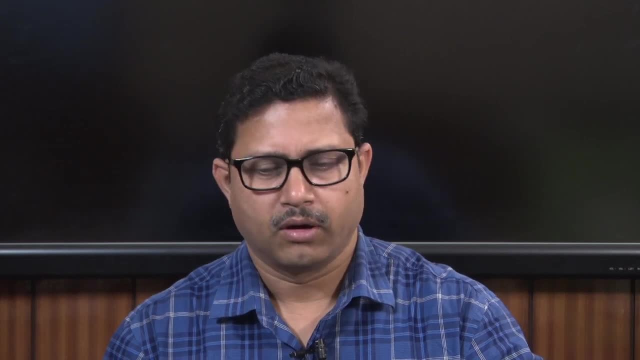 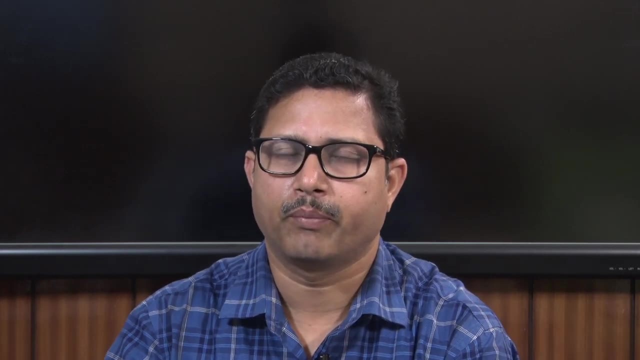 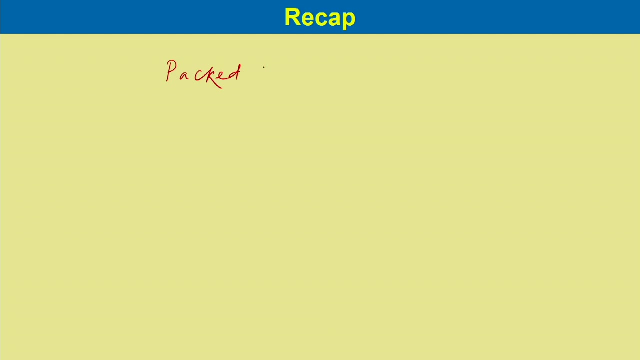 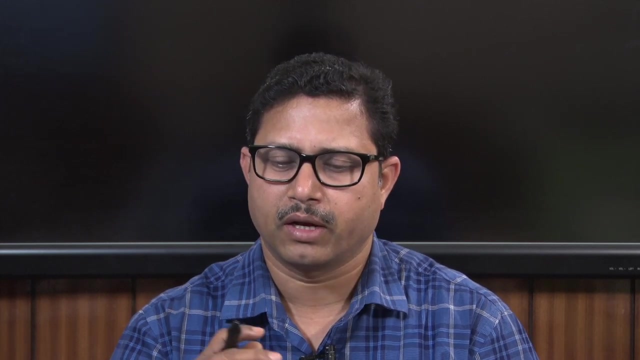 a brief recap on our previous lecture. On our previous lecture we have mainly considered one important topic. We have discussed packed tower distillation. In the packed tower distillation we have seen what are the types of liquid mixtures we can use for packed tower distillation. 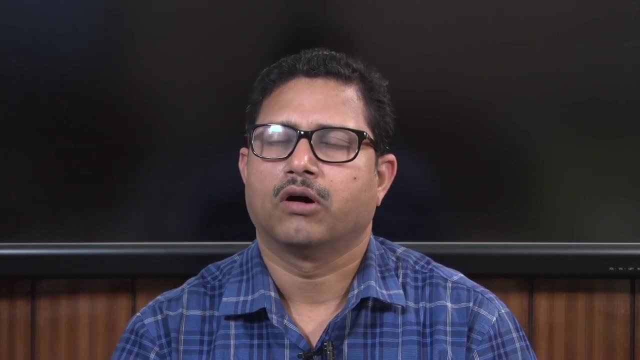 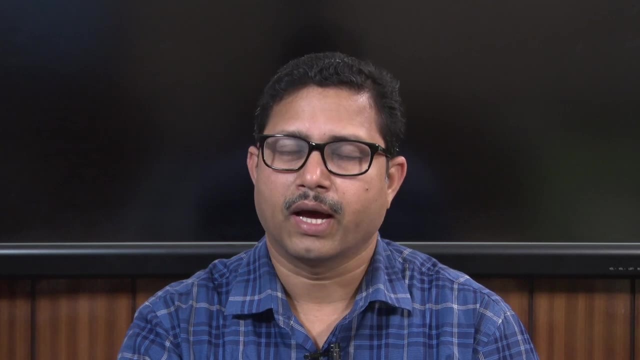 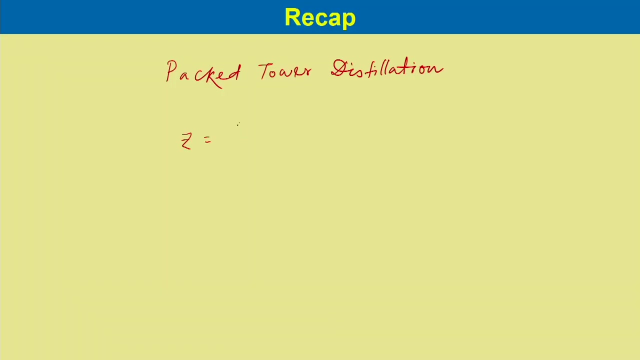 And what would be the conditions of those liquid mixtures. At the same time, we have considered to calculate the height of the tower required, that is z. 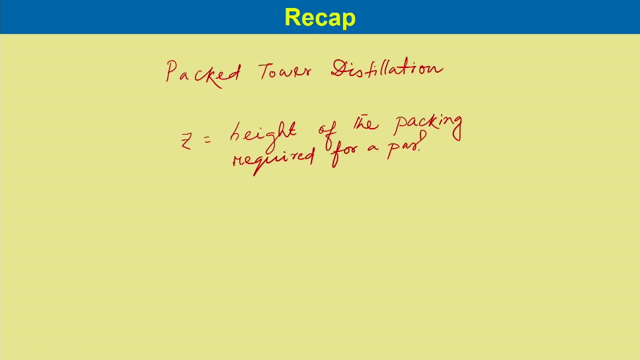 and we have seen that it is similar to the packed tower absorption operations. We have considered the packed tower design based on the volumetric mass transfer coefficient. 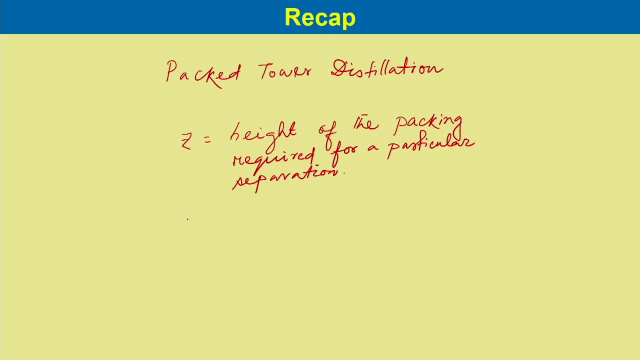 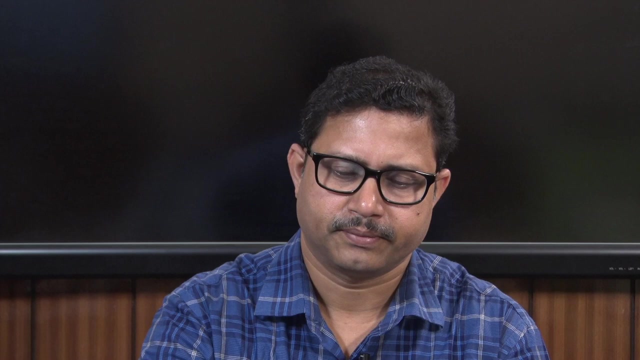 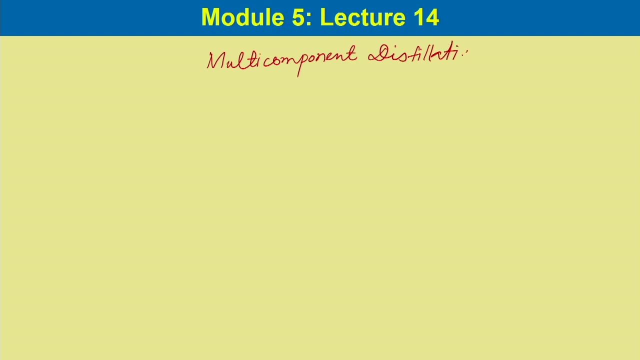 both in the liquid phase as well as in the gas phase, that is, k y a dash and k x a dash. So in this lecture we will consider multicomponent distillation, under which we will mainly focus on bubble point and dew point calculation. 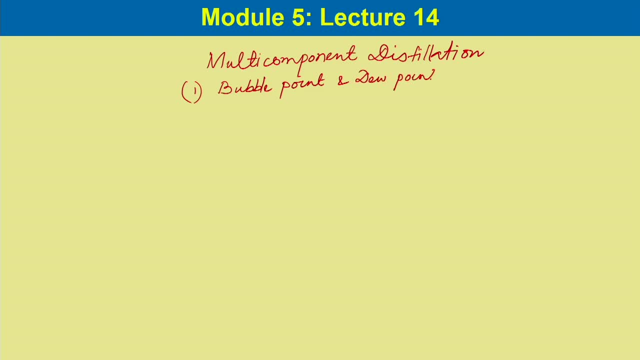 The second thing we will consider is the multicomponent flash distillation. Then we will consider multicomponent batch distillation. We will also consider to find out the minimum number of plates that is a total reflux. So then we will consider minimum reflux and finally we will consider the approximate. 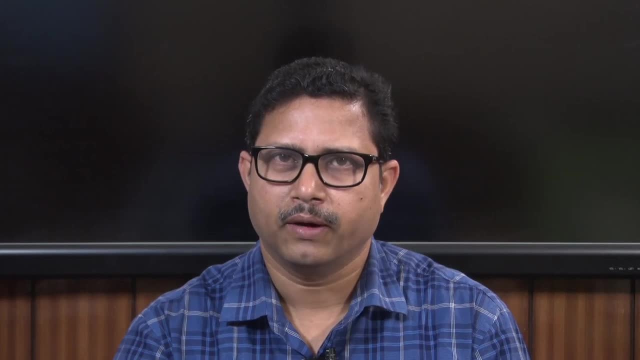 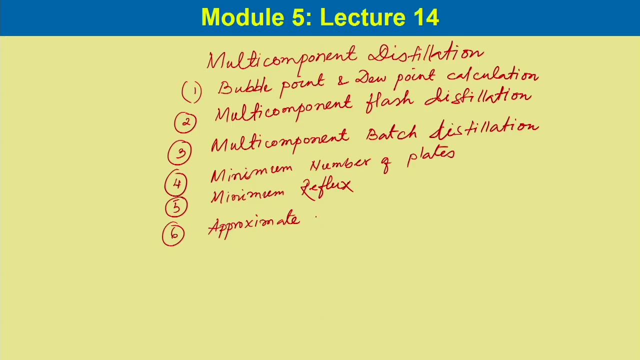 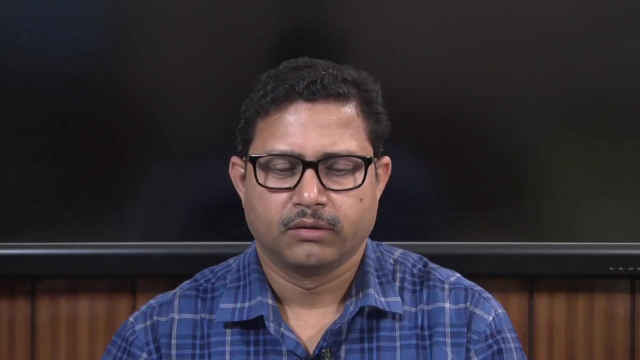 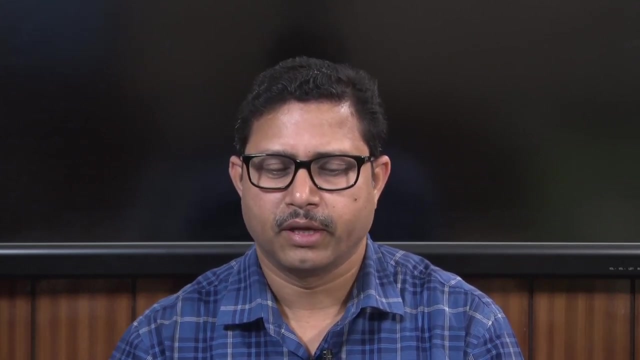 method or under root method to calculate the composition stations of the tower and the number of trays required. So multi component distillation. So there are three component systems, at least more than two component systems. If it is three component systems, then graphical treatment. 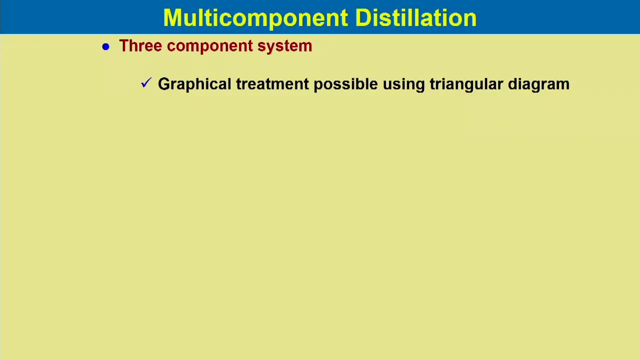 is possible using triangular diagram If more than three components are there. in that case, graphical treatment is very complicated. For practical application, liquid phase may be assumed. ideal Raoult's law may be applicable, and equilibrium data can be obtained from pure component data. 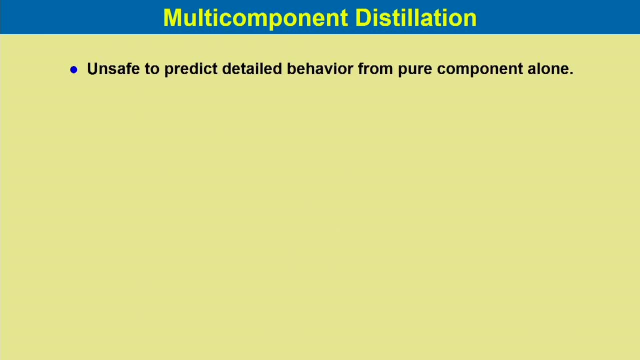 Now it is unsafe to predict detail behaviour from pure component alone, So digital computer is helpful for data analysis to predict detail behaviour. The overall approach To solving multi component problems is the same in many respect as those described for binary systems. So if we consider overall approach for the solution of the multi component, 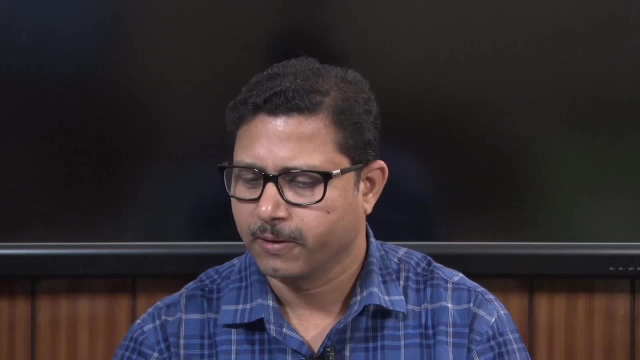 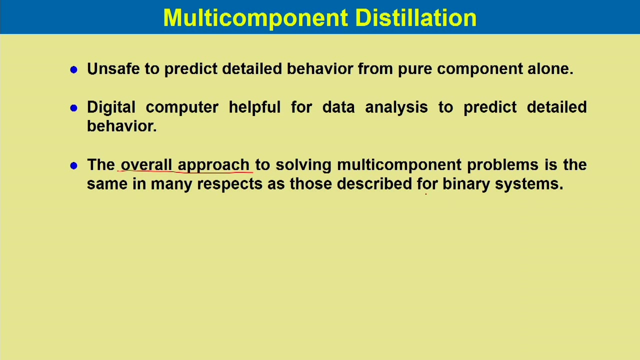 systems or for the design of the multi component systems. in many respect it will be similar as those for the binary system. There is one mass balance for each component and enthalpy balances are similar to those for binary case. So what we can see here in this case the mass balance. 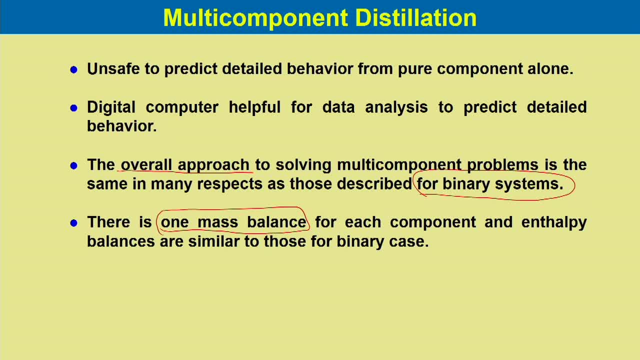 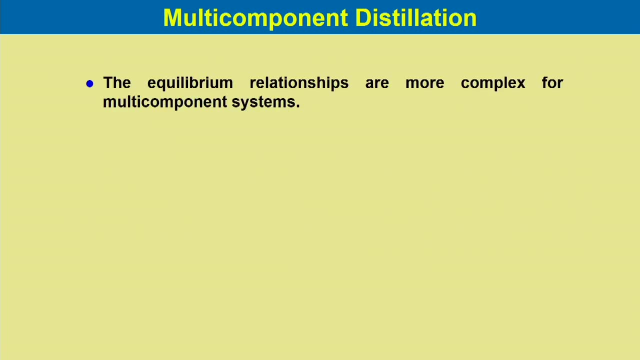 for each component will be one. for each component we will have one mass balance and the enthalpy balance would be similar to those for the binary case. The equilibrium relationship are more complex for multi component systems. In particular, the identity of the most volatile component may change with temperature of the systems. 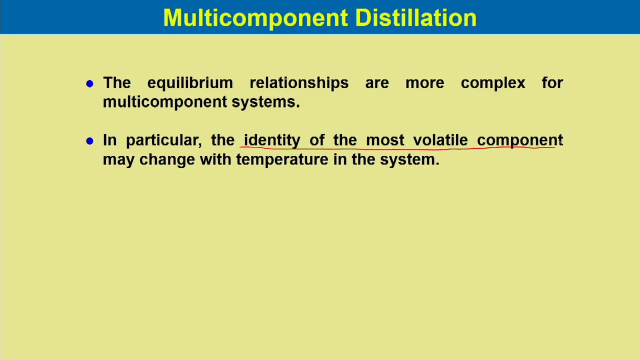 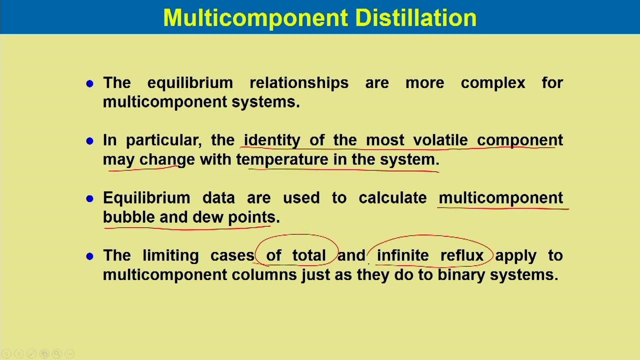 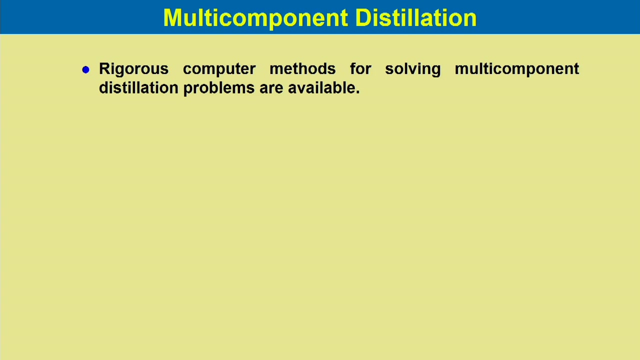 Please note that the identity of the most volatile component. In this case also, we can apply the limiting cases for total reflux and infinite reflux, and that would be similar as we do for the binary systems. Now, rigorous computer methods for solving multi component distillation problems are. 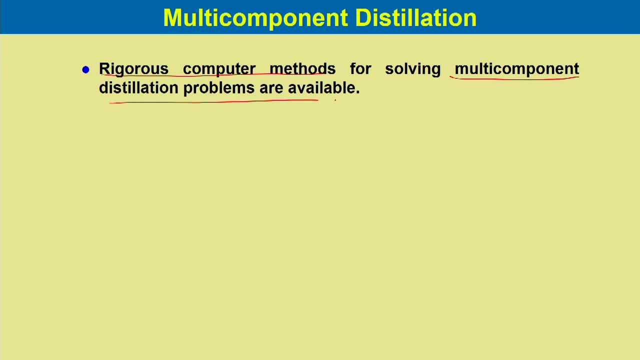 available, But the approximation of the total reflux is not possible. The simplified or shortcut methods described here are common for preliminary design, examining the relationship between the design parameters and process, synthesis, etcetera, Although there are rigorous method computer methods available for the multi component distillation problems. 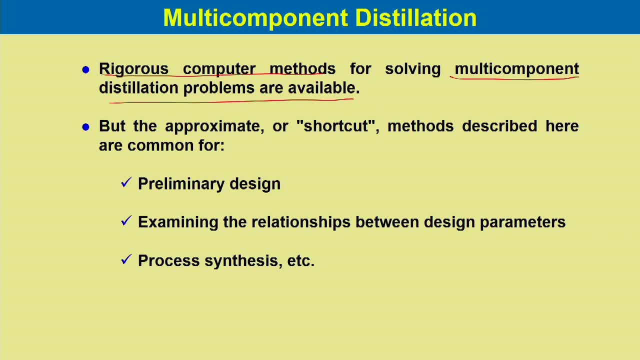 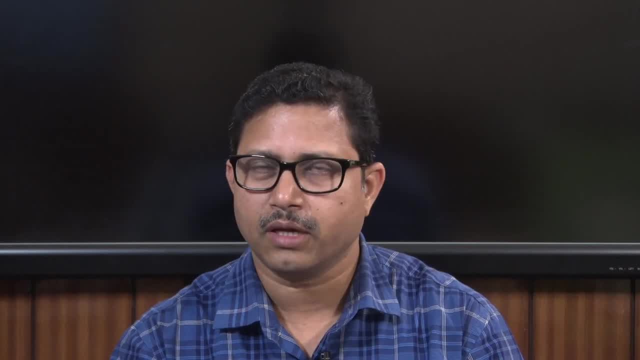 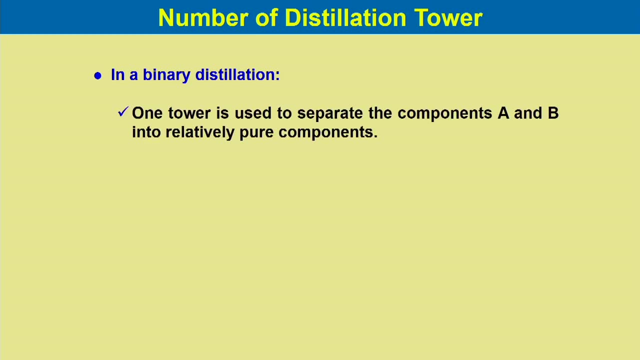 but approximate method can be helpful for preliminary design, design, examining the relationship between the design parameters, process synthesis and so on. Now, number of distillation tower. in a binary distillation, as we know, one tower is used to separate the components A and B into relatively 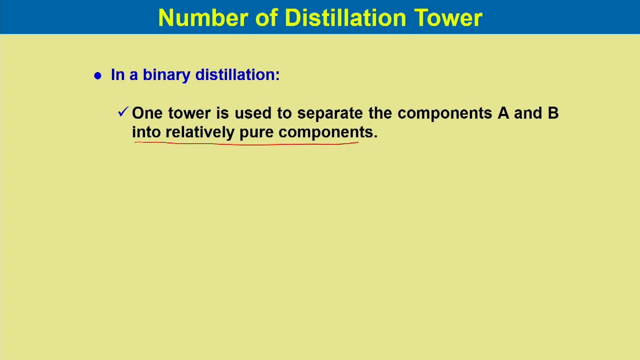 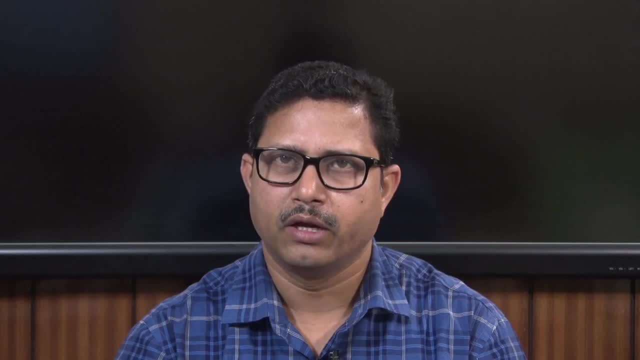 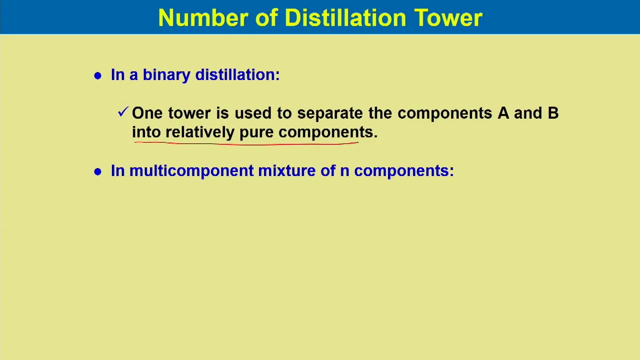 pure components. So we generally use one tower having several trays which can separate the binary component into fractions, relatively pure component fractions. But in multi component mixture of N components we need N minus 1 fractionators which are required for the separation. that means if we have 3 component mixture then N is equal. 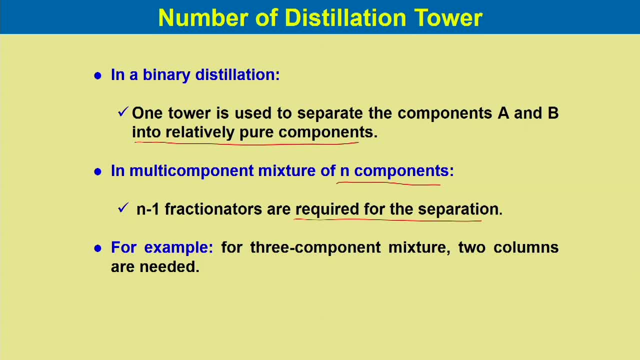 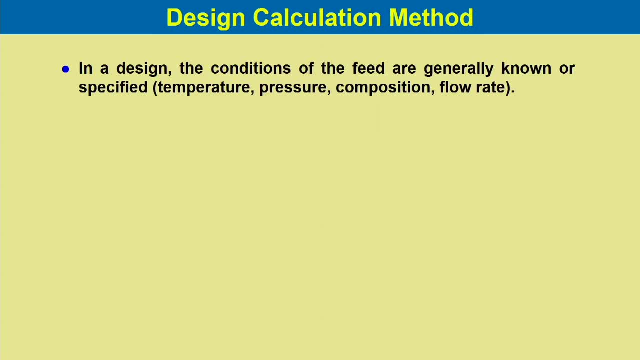 to 3, so we need N minus 1 fractionators. that means two columns are needed In a design. the conditions of the feet are generally known or specified. that means the temperature, pressure, composition and flow rate. These conditions of the feet are generally known or it should be specified at the beginning. 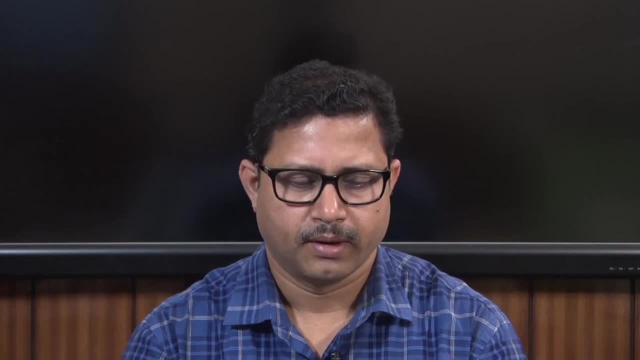 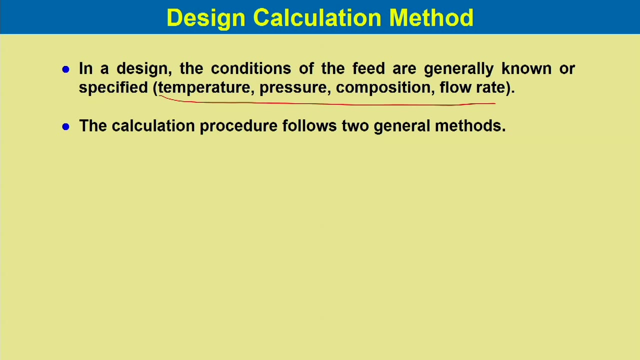 of the design. The calculation procedure follows two general method. Let us consider what are those. Method 1, the desired separation or split between two of the components is specified and the number of theoretical states, The number of theoretical stages, is calculated for a selected reflux ratio. So the split. 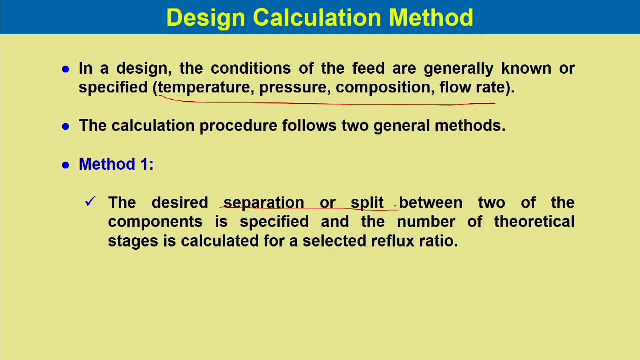 or separation between the two components has to be specified, and then we calculate the number of theoretical stages based on a selected reflux ratio. It is clear that with more than two components in the feet, the complete composition of the distillate is calculated based on the 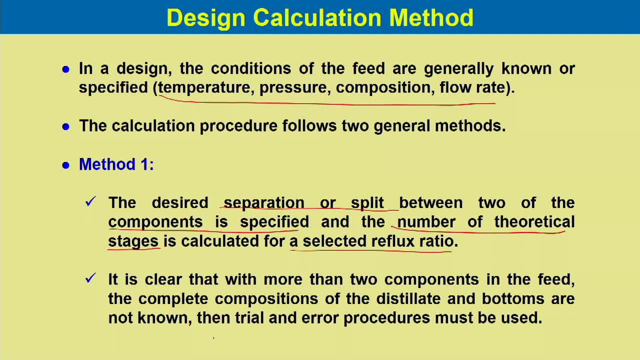 number of stage and the bottoms are not known, Then trial and error procedure must be used. This is very clear for more than two component systems in the feet. the complete composition of the distillate and bottoms are not known. So we should follow the trial and error procedure. 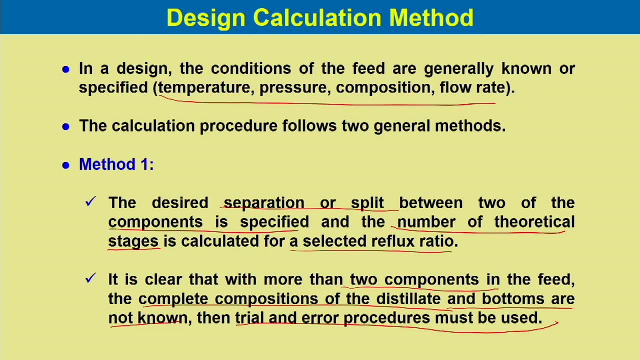 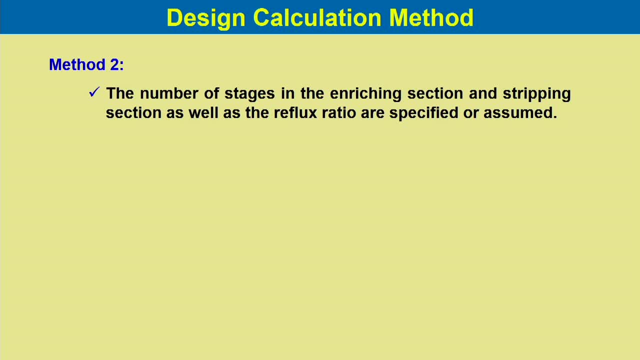 to calculate the compositions: Method 2, the number of stages. Method 2, the number of stages. stages in the enriching section and stripping section, as well as the reflux ratio are specified or assumed. So both section- enriching section and stripping section. in addition to that, 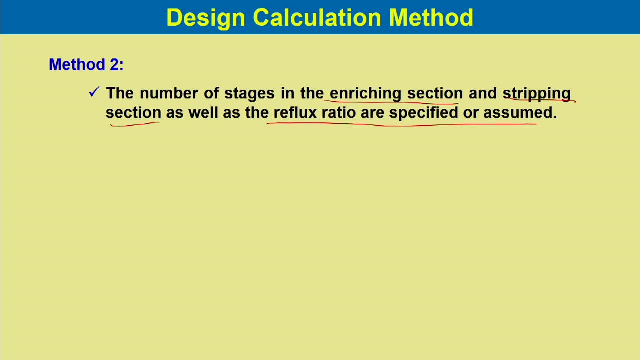 the reflux ratio has to be specified at the beginning. The number of component is calculated using assumed liquid and vapour flows and the temperature for the first trial. So what? we are- assuming liquid and vapour flows and the temperature for the first trial. This. 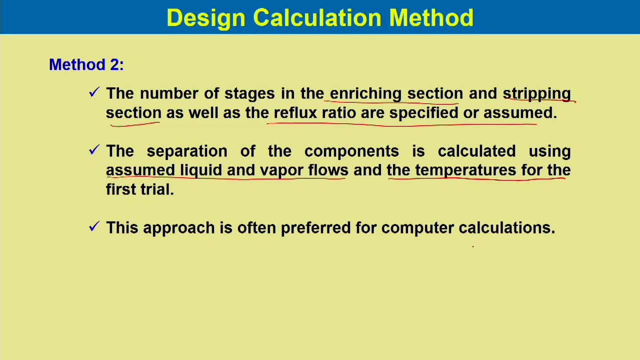 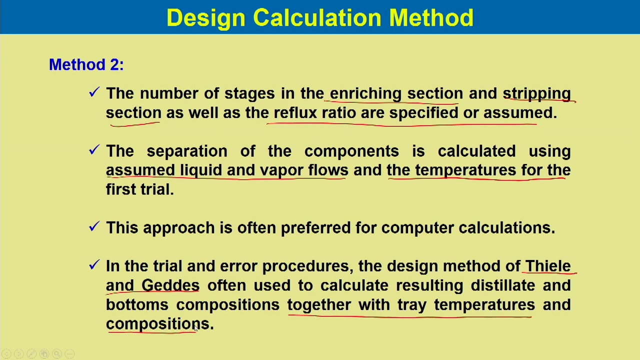 approach is often preferred for computer calculation. In the trial and error procedures the design method of Thiele and Geddes is often used to to calculate the resulting distillate and bottoms composition, together with tray temperature and compositions- Now equilibrium in multicomponent systems. 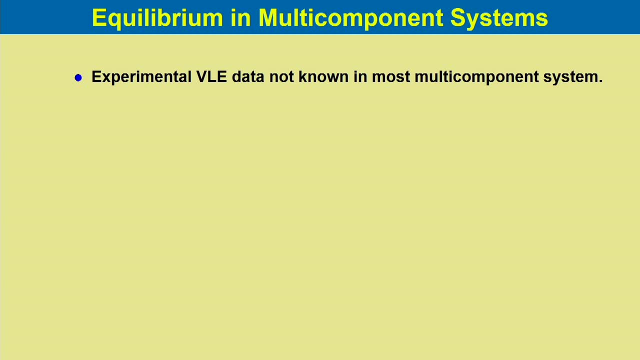 Experimental VLE data not known. in most multicomponent systems, generally computed from available equations or correlations, Ideal behaviour may be assumed So that we can apply the Raoult's law. Hydrocarbons of a homologous series form nearly.